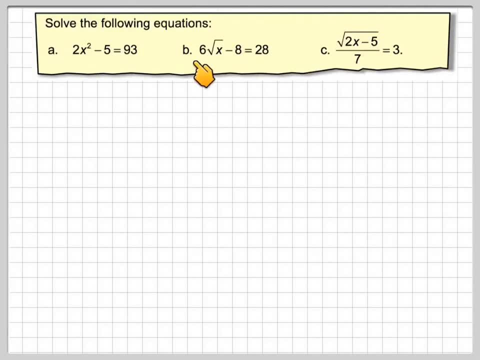 Hi, this video is about solving equations which either have powers in them or roots in them. So we've got solve the following equations: which is 2x squared minus 5 is equal to 93.. 6 root x minus 8 is equal to 28.. The square root of 2x minus 5 over 7 is equal to 3.. 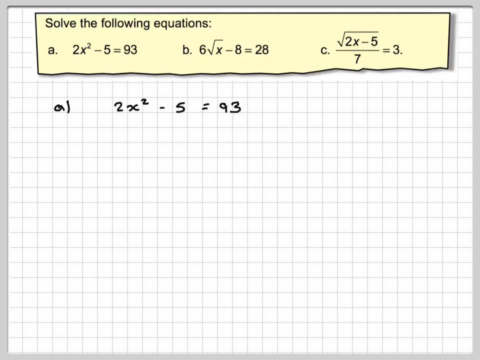 So writing down the first one, we've got: 2x squared minus 5 is equal to 93.. Now, solving equations, it's all about balance and doing opposite. So we've got to take 2x squared, take 5.. Now the opposite of taking 5 is to add 5 to both sides. 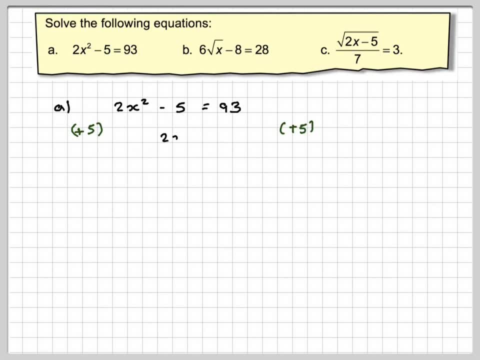 So if we add 5 to 2x squared minus 5, we just get 2x squared, And if we add 5 to 93, we're going to get 98. So we've got two times here. so the opposite of multiplying by 2 is to divide by 2.. 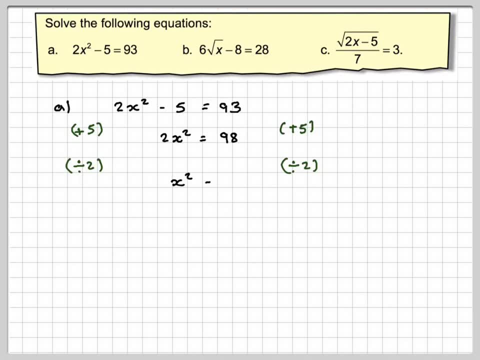 So we end up with x squared on this side and then 98 divided by 2 is 49. Now the opposite of squaring is to take the square root. So the square root of x squared is x and the square root of 49 is plus or minus 7.. 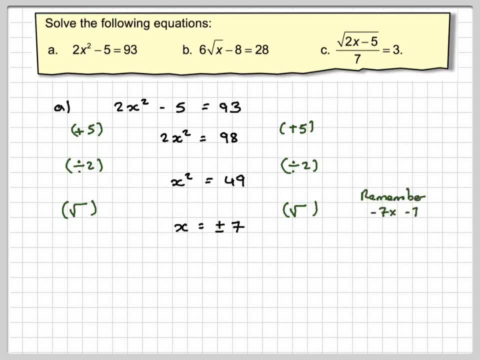 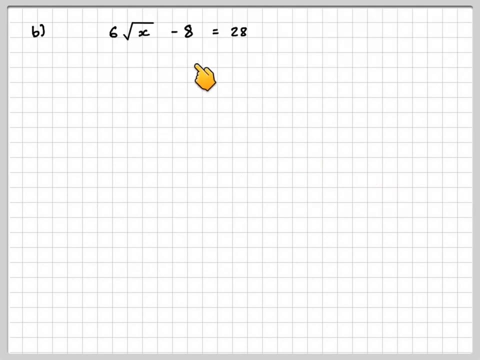 Now it's plus or minus 7, because if we do minus 7 times minus 7, we do get plus 49.. So there's two possible answers: x is minus 7, or x is equal to 7.. Right now we have 6 root x minus 8 is equal to 28.. 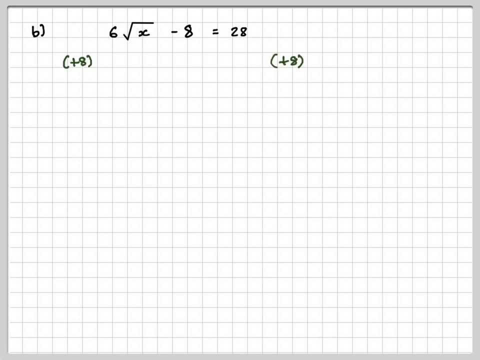 It's the same thing. Obviously I'm subtracting. 8 is to add 8 to both sides, so we get 6. root x is equal to 28 plus 8, which is 36.. 6 times the opposite of multiplying by 6 is to divide both sides by 6.. 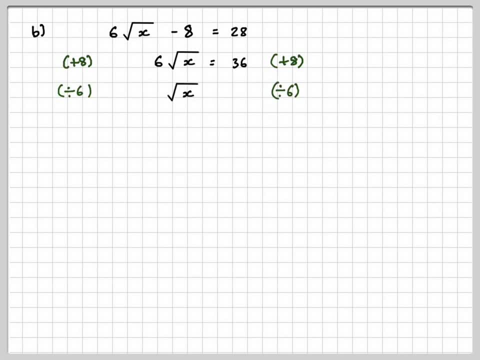 So this side we get root x and 36 divided by 6 is 6.. So the opposite of doing the square root is actually to square. So if you square square root and then square, you're just left with x, And then if you square 6,. 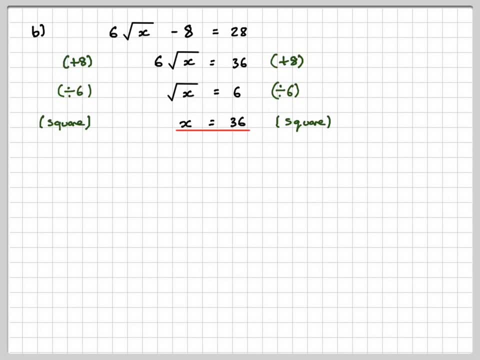 you get 36, which is the final answer. Part c: square root of 2x minus 5 over the 7. The square root's only over the numerator, So the first step would be to multiply both sides by 7..